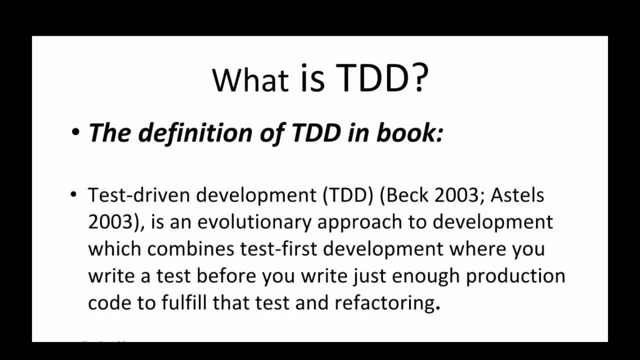 So let's look at the definition of TDD. in book Baker, the author of Test-Driven Development, said TDD is an evolutionary approach to development which combines test-first development- where you write a test before you write just enough production code to fulfill that test- and refactoring. 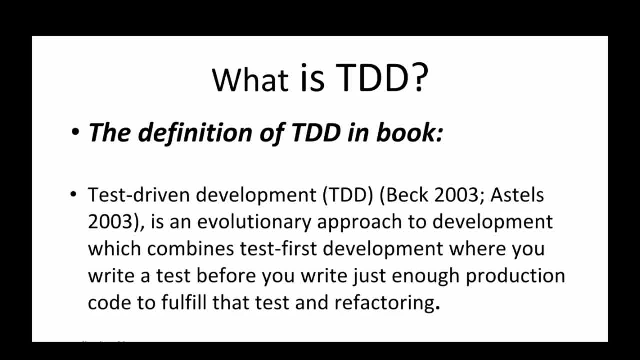 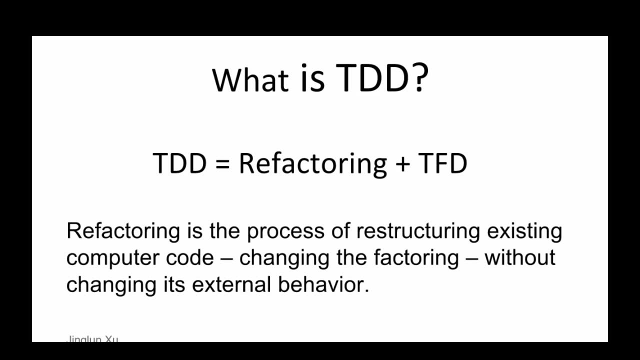 Here. the author mentioned that TDD is an evolutionary approach to development where you write just enough production code to fulfill that test and refactoring. I would like to describe TDD with this simple formula: TDD is equal to refactoring plus TFD. 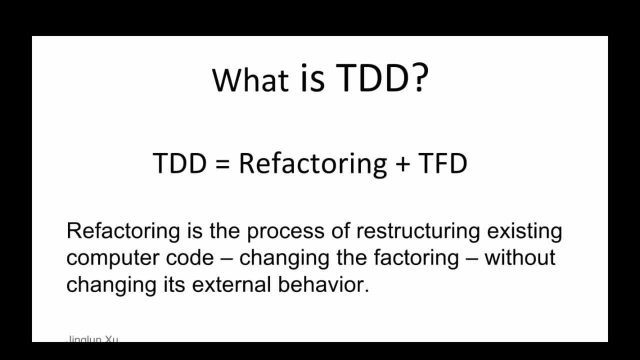 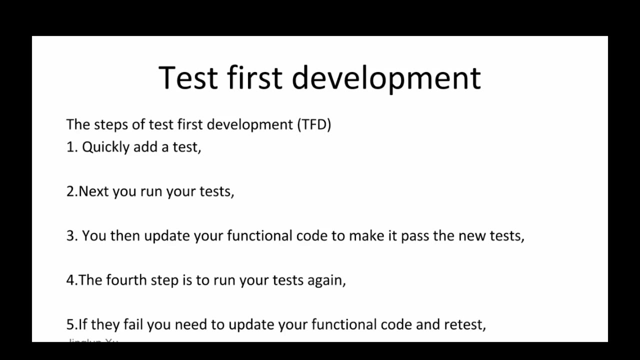 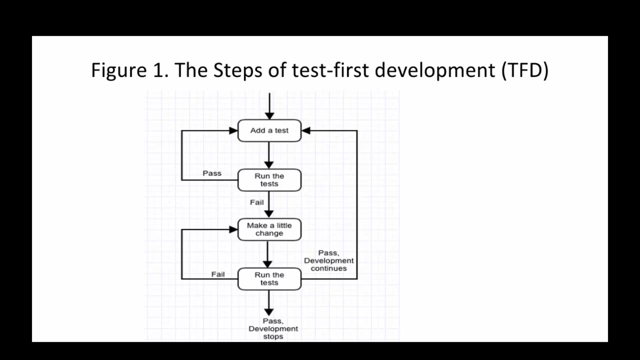 So refactoring is the process of restructuring existing computers, the existing computer code, changing the factoring without changing its external behavior. So let's look at the steps of TFD. The first step is to quick-add a test. basically just enough code to fail. 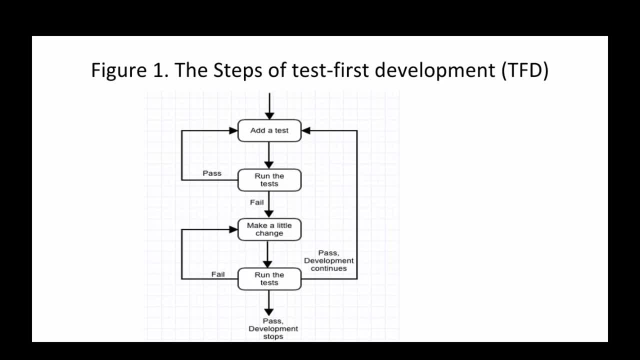 Next, you should run your tests to ensure that the new test does in fact fail. You then make a little change and update your functional code to make it pass the new test. The fourth step is to run your tests again. If they fail, you need to update your functional code and re-test. 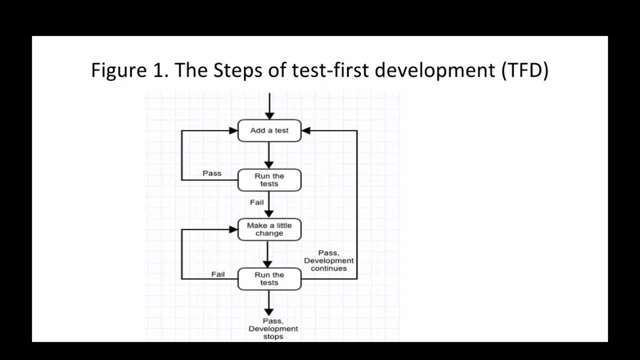 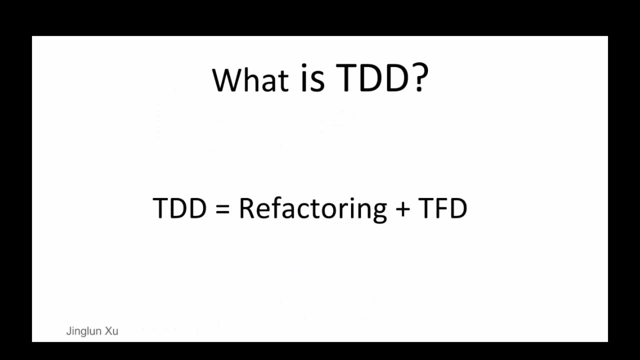 Once the tests pass, the next step is to start over. You may first need to refact any duplication out of your design as needed, turning TFD into TDD. So that's it, Thank you. So TDD completely turns traditional development around. 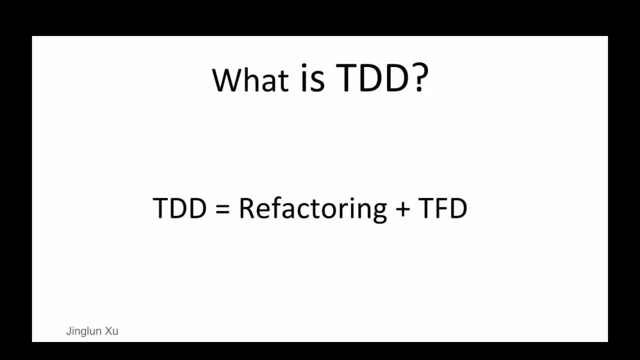 When you first go to implement a new feature, the first question that you ask is whether the existing design is the best design possible that enables you to implement that functionality. If so, you proceed with a TFD approach. If not, you refactor it. 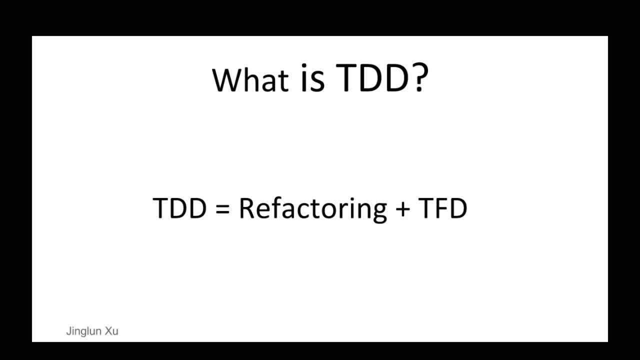 If not, you change the portion of the design affected by the new feature, enabling you to add that feature as easily as possible. As a result, you will always be improving the quality of your design, thereby making it easier to work with in the future. 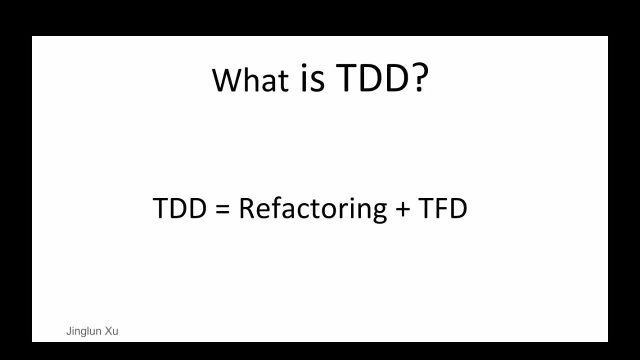 Instead of writing functional code first and then your testing code- as I said, As an afterthought, if you write it at all- you instead write your test code before your functional code. Furthermore, you do so in very small steps: one test and one small bit of corresponding functional code at a time. 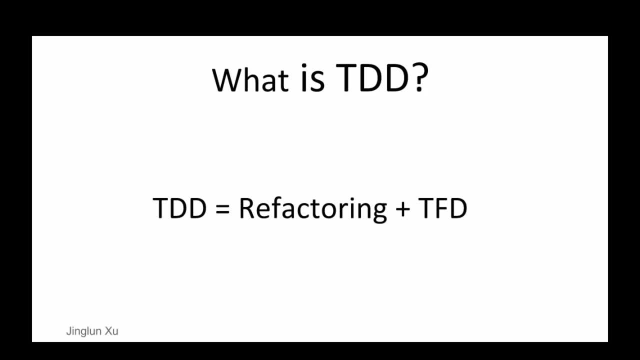 A programmer taking a TDD approach refuses to write a new function Until there is first a test that fails because the function isn't present. In fact, they refuse to add even a single line of code until a test exists for it. Once the test is in place, they then do the work required to ensure that the test should now pass it. 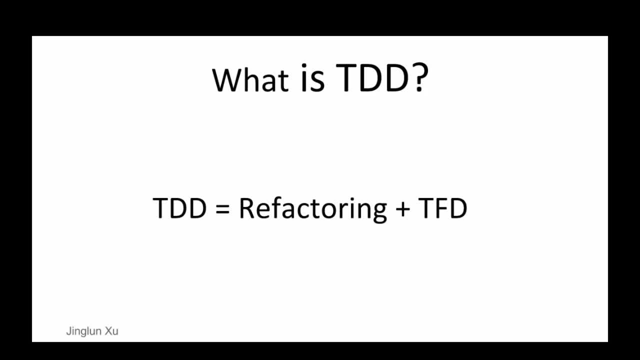 This sounds simple in principle, But when you are first learning to take a TDD approach it proves requires great disassembling because it is easy to slip and write functional code without first writing a new test. One of the advantages of pair programming is that your pair helps you to simplify your programming. 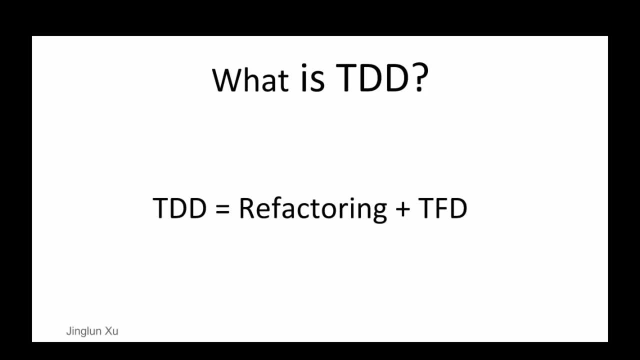 It helps you to stay on track. Next, let's look at the two levels of TDD. The first level is acceptance TDD. We call it ATDD. With ATDD, you write a single acceptance test, or behavioral specification, depending on your preferred terminology. 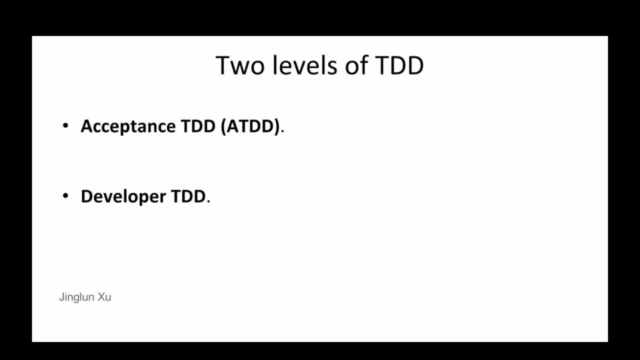 and then just enough production functionality code to fulfill that test. The goal of ATDD is to specify detailed executable requirements for your solution on a just-in-time basis. ATDD is also called behavior-driven development, Then developed TDD. you write a single development test. 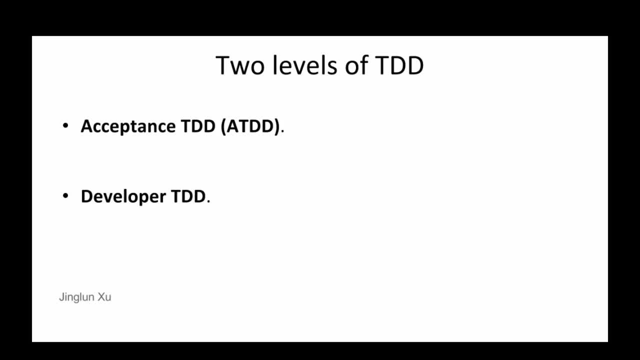 Sometimes inaccurately refilled as a unit test and then just enough production code to fulfill that test. The goal of developed TDD is to specify a detailed, executable design for your solution on a just-in-time basis. Developed TDD is also simply called behavior-driven development. 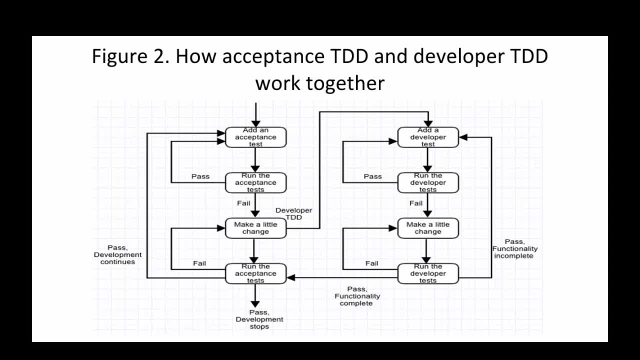 In the previous lecture we talked about the development of TDD. Now let's look at theudd. OK, we write game test by am passing test d left. However, we can write an dichalect test by approach vend stars with this example. 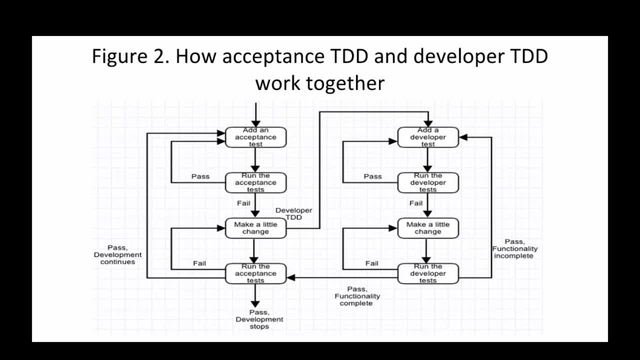 Another condition of 저기자1 is testing this Ben to to it. so then, This in turn requires you to iterate several times through the write test. write projection code. get it working cycle at the developed TDD level. Note that this figure: 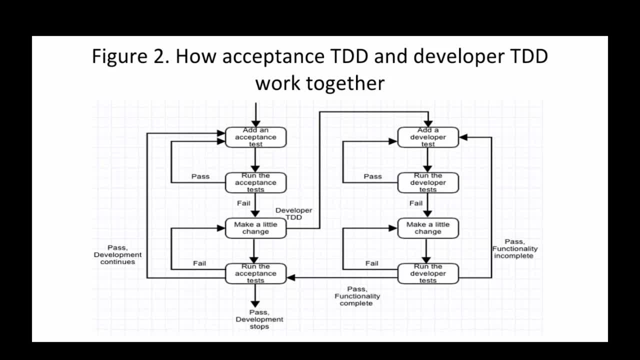 assumes that you are doing both, although it is possible to do either one without the other. In fact, some teams do developed TDD without doing ATDD, although if you are doing ATDD, then it's pretty much certain you are also doing developed TDD. 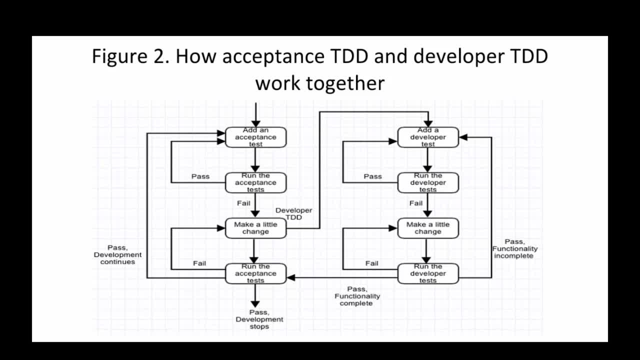 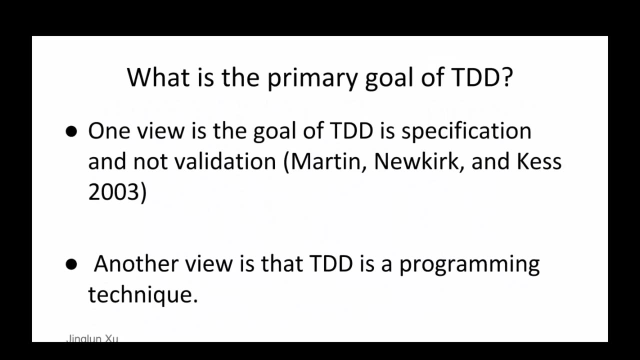 The challenge is that both forms of TDD require practitioners to have technical testing skills, These skills that many requirement professionals often don't have. And next, What is the primary goal of TDD? One view is that the goal of TDD is a specification, and 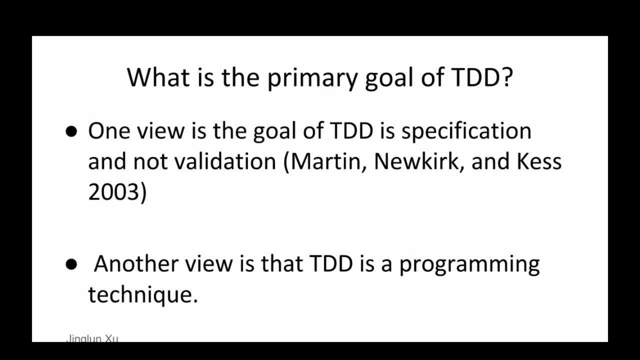 not a validation. In other words, it's one way to think through your requirements or design before you write your functional code, implying that TDD is both an important agile requirement and agile requirement. Another view is that TDD is a programming technique, As many people like to say. 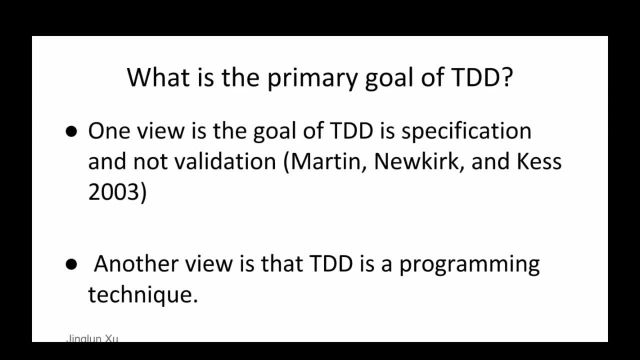 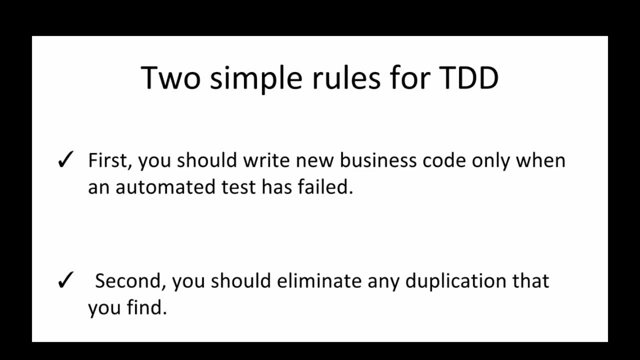 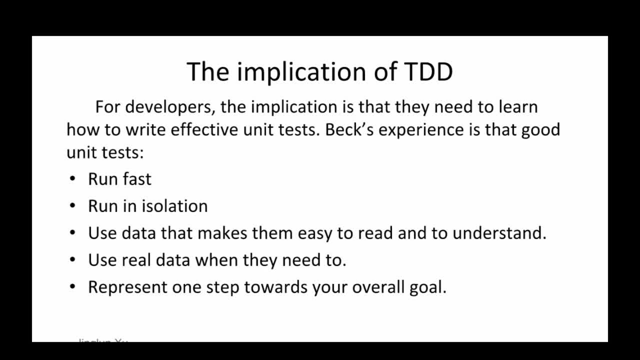 The implication of TDD is that they need to learn how to write effective unit tests, should use real data when they need to. At last, it should represent one step towards your overall goal. Okay, that's my part. Let's welcome He Yi to introduce the. 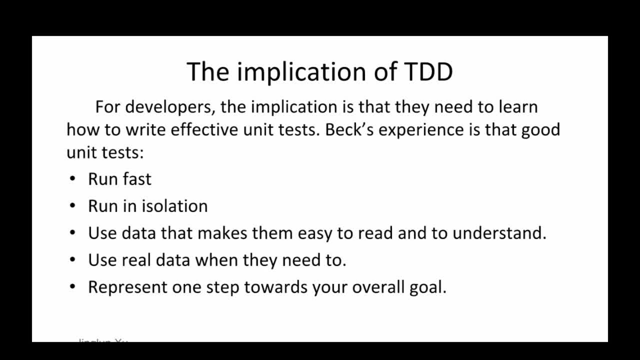 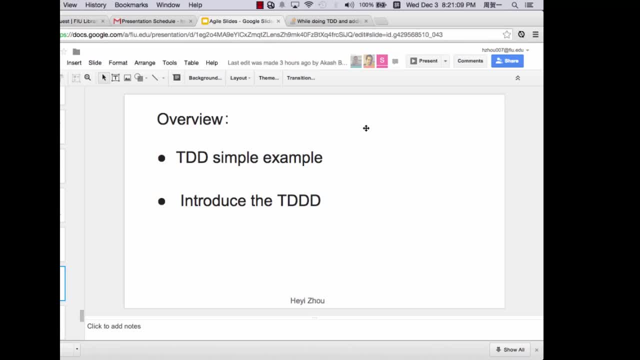 next part. Hello everyone, I'm He Yi. The first part has been done. He has introduced the set of tests for the development, and then what is TDD, and then the level of TDD and what is the primary goal of TDD. The second round: 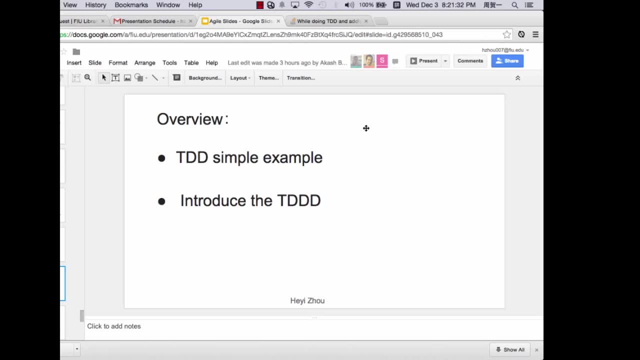 The second part. I want to introduce it from two points. One point is TDD. simple example and introduce TDDD. TDDD full name is TDD for Relational Database. What is TDDD? In my opinion, TDDD means that Methods of Development, Development of Design. 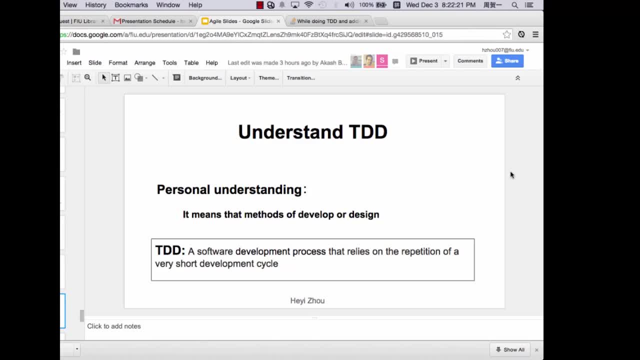 Some people think it's TDD. Some people think it is a software development process that relies on the repeating of a very short development cycle and TDD general processes. If you guys saw the wiki, it tells the TDD have three parts. 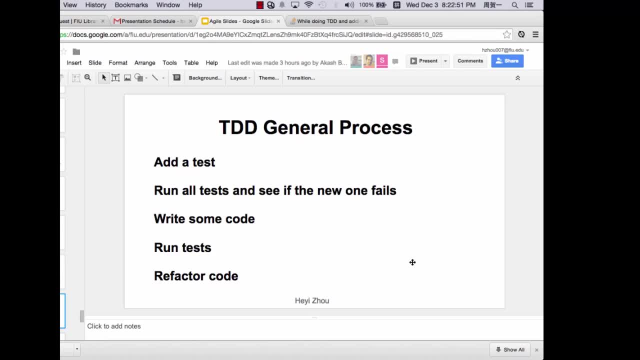 DDD has five processes: either test, run or test and see if the new one is false. Write some code, run test, refactor code. But I think TDD general process have three processes. The write processes is the green processes. 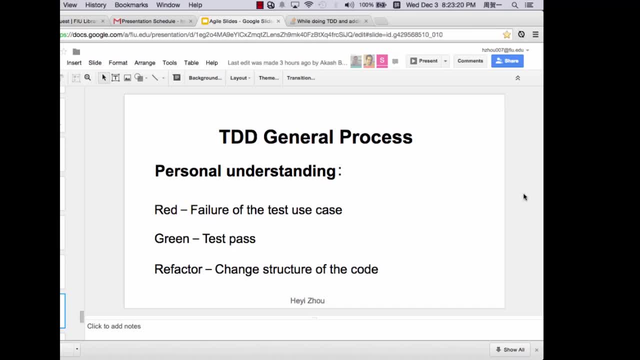 and the factory process. The red process means the future of the test use case And the green process means the test path is green, Color is green And the third part is the change structure of the code. Let me give you an example to understand the TDD. 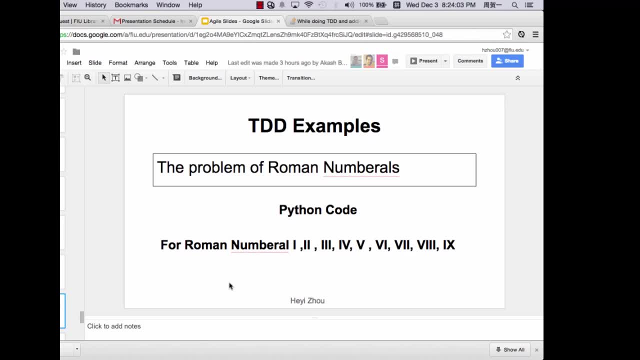 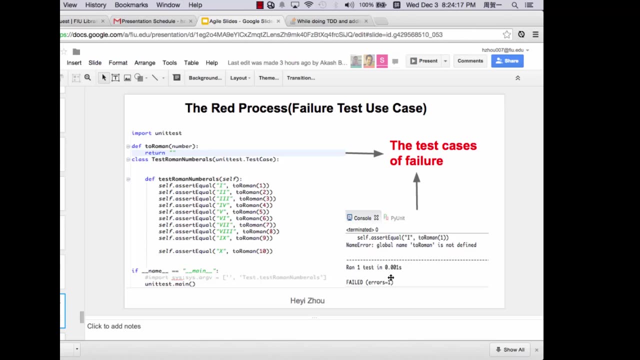 Everyone knows the problem of Roman numbers. For Roman numbers there are thousands of numbers. If I, If I need to test 10 numbers first, I will create the function, The following: I will give you an example for TDD. I give the problem of Roman numbers to the TDD. understand the TDD. 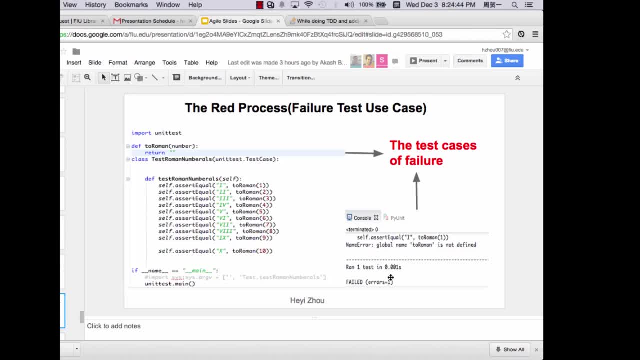 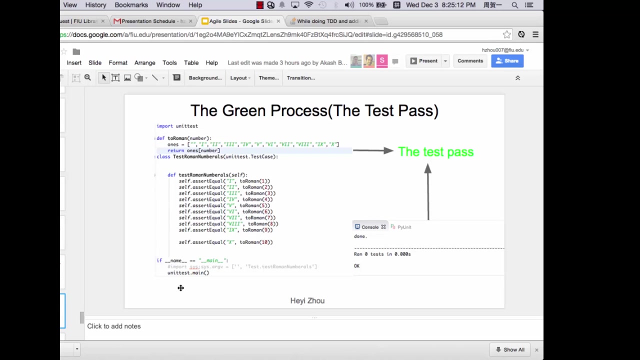 If I just do test 10 number first, we don't need to give the statement. the process is the test case of the future, The future is necessary, The future is necessary. And the second step, The next step: we need to create the function of the statement. 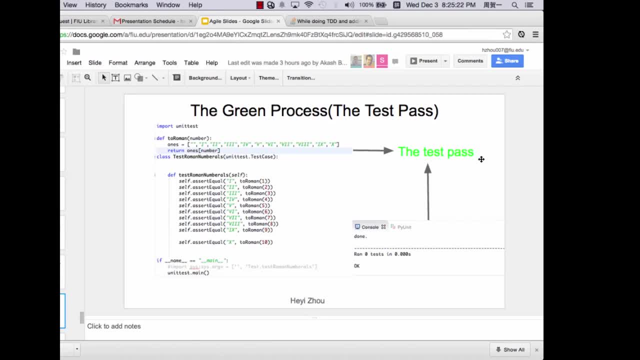 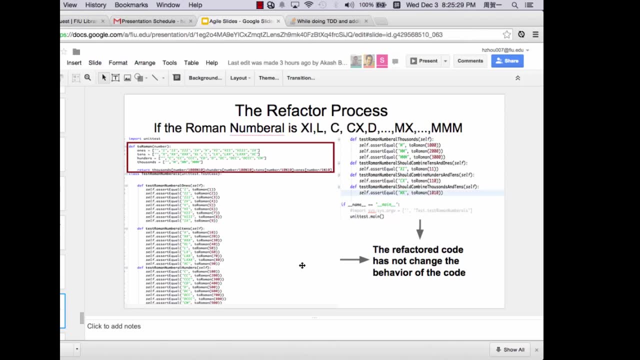 And this path is, This process is a test path. And then if we have, If we have thousands of numbers for the code and we need to refactor, code has not changed the behavior of the code. This process, This process is a refactor process. 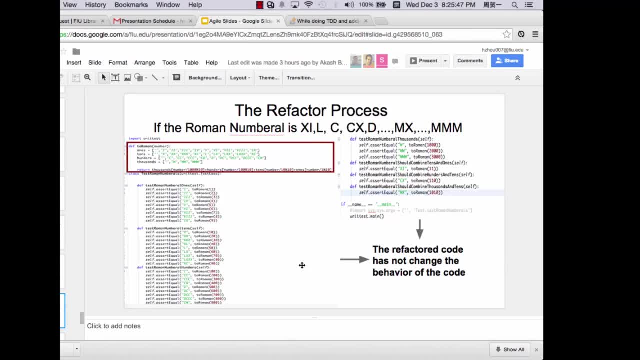 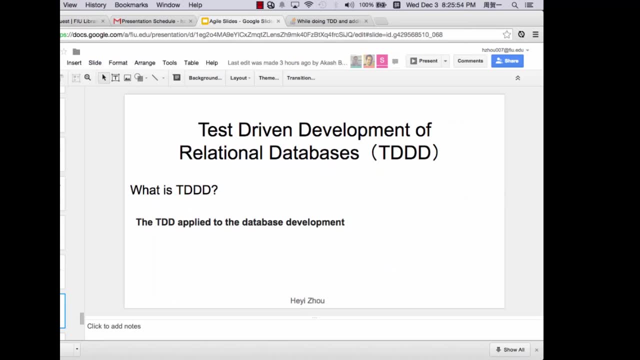 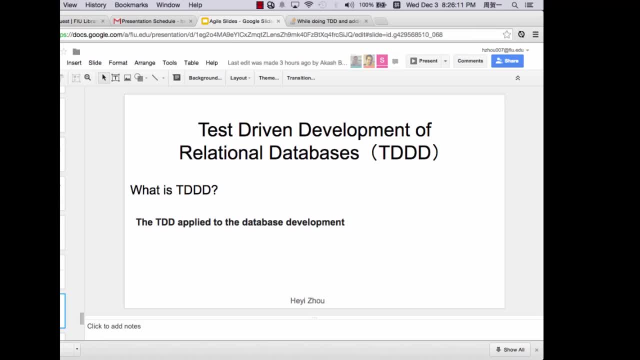 And next we need to, And next we need to, And next I want to talk about TDDD. TDDD full name is test driven- development of a relational database. What is TDDD? The TDDD means TDD applied to the database development. 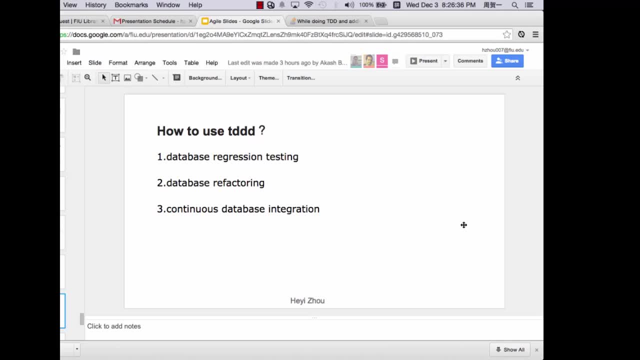 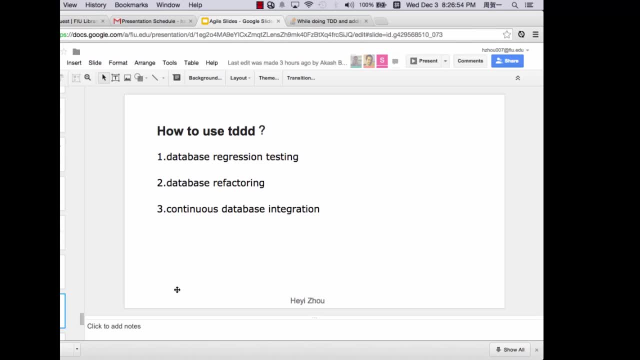 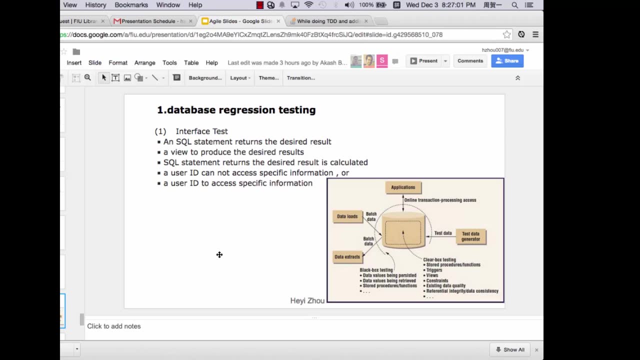 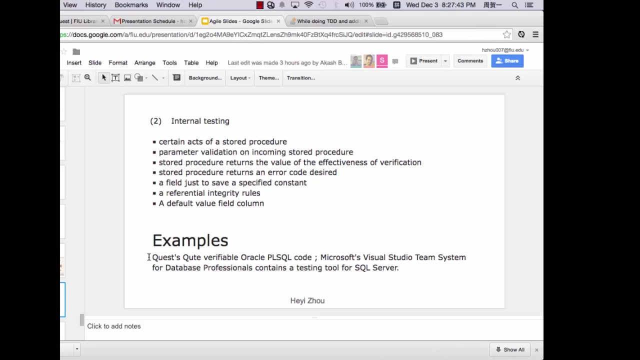 the continuous database Test, the database rejection, have two processes: Interface, the test- Look at the picture. There are three. there are four parts focused on database: The applications, date loads, date extracts and the test date generator. The two part is internal test. 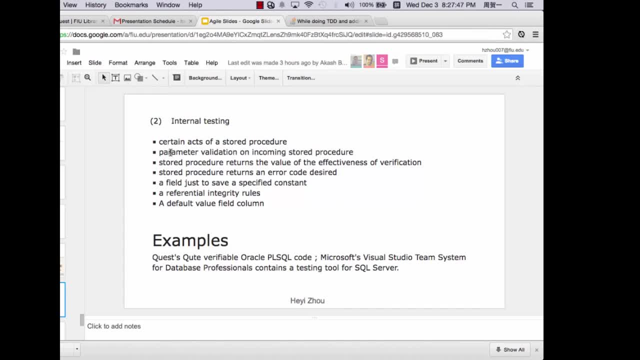 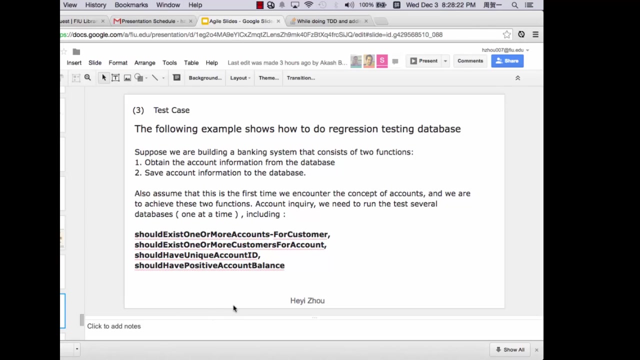 The internal test, however, contain uncertain acts of stored produce. Timer evaluation on incoming stored produce And the store producer returns the value of the effect, Effectiveness of verification and so on. The following give you an example. This example shows how to do rejection testing database. 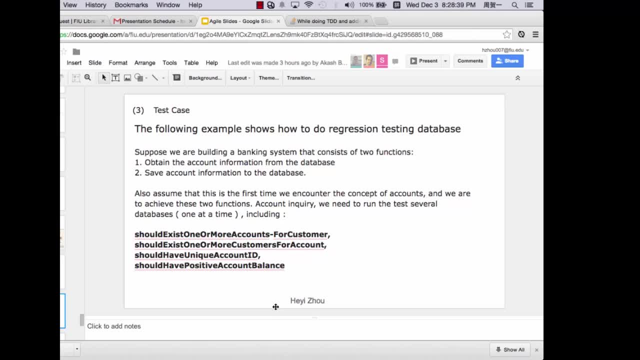 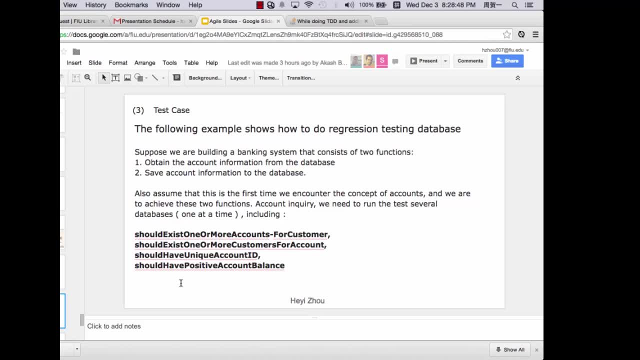 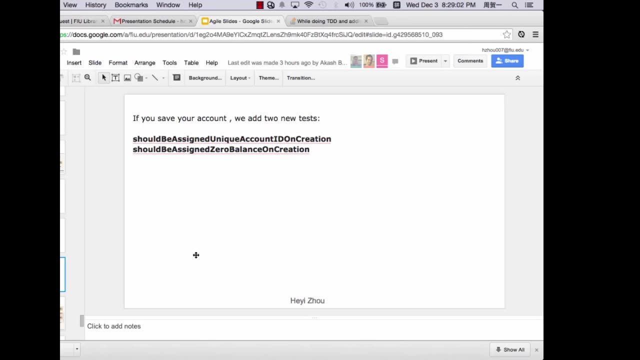 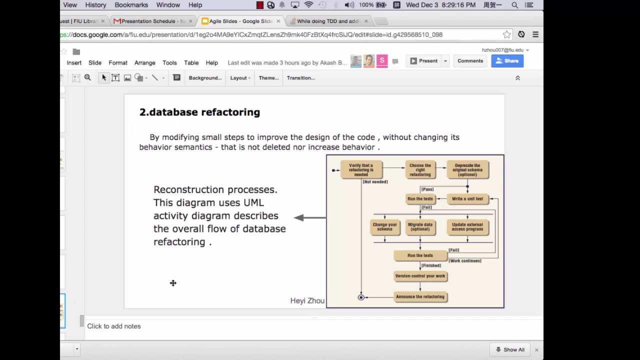 And this is a function for the example, If you save your account, we need to add two new tests. And this is two function for adding new tests And the database refactoring. Database refactoring means, by modifying small steps to improve the. 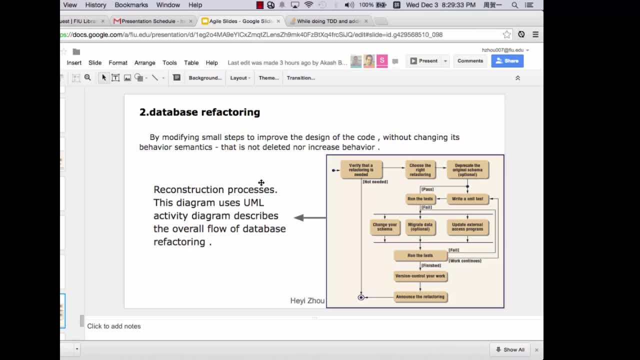 design of the code without changing its behavior symbols. then it is not deleted or increase behavior. Look at the picture. First step: we can verify that refactoring is needed and go through, choose the right refactoring and then go through and operate the original. 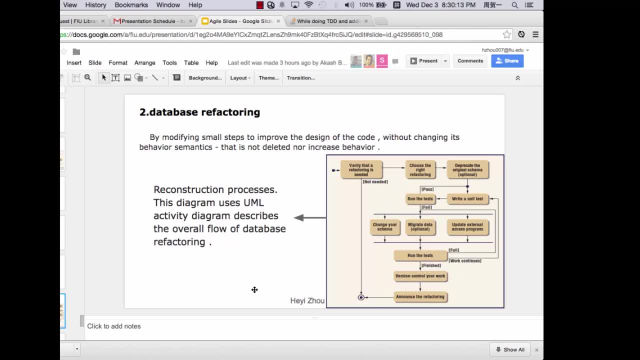 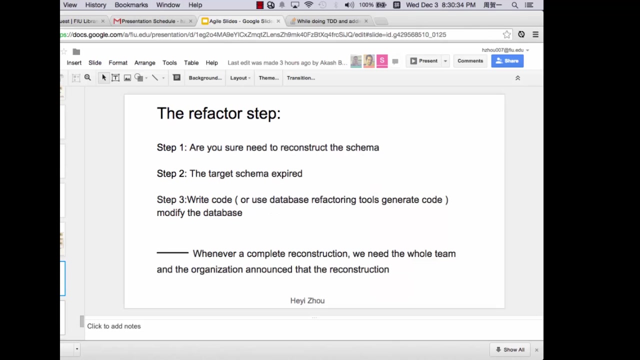 schema and so on and so on. The construction process is: this diagram uses UML. activity diagram describes the overall flow of database refactoring. The refactor step for relational database have three steps. The first one is: are you sure need to reconstruct of the schema? 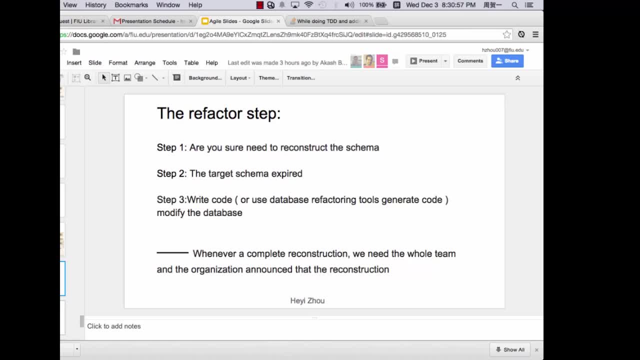 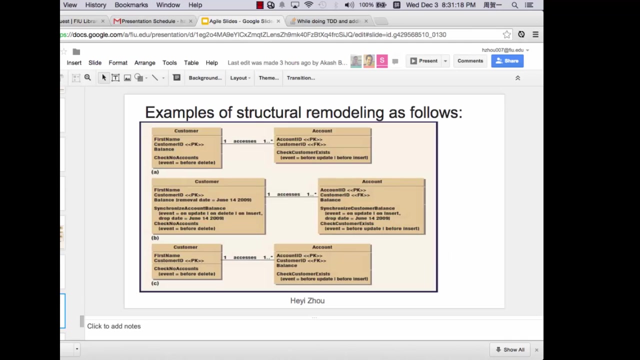 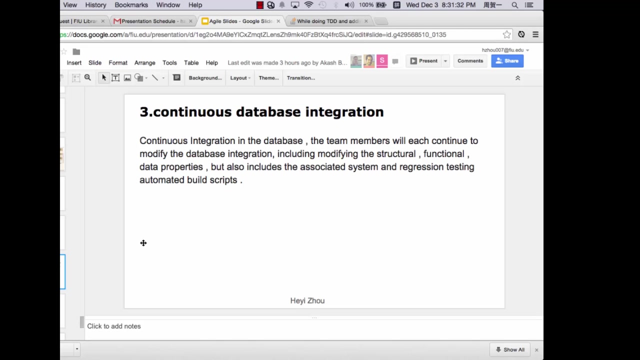 and the target schema, SW-Expand and then RedCode. Some people think it is a good idea to Whenever a complete reconstruction we need. the whole team and the organization announced that reconstruction. This picture shows that structural remodel as follows: Continuous database integration. 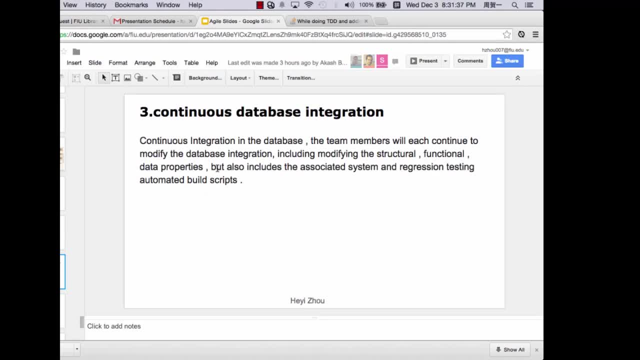 Structural database integration means that the team members will each continue to modify the database integration, including modifying the structural functional database properties, but also includes the society system and the regression testing automated. For example, all the data in the database is used to chili process. 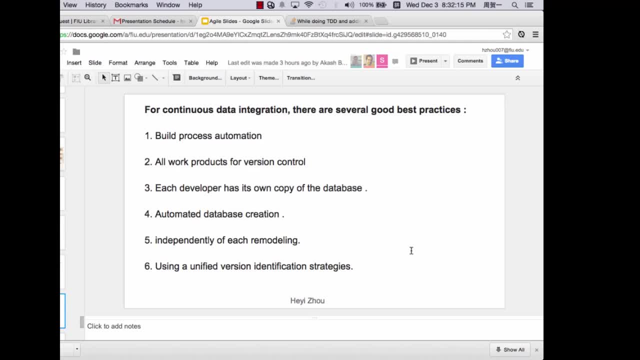 So the entire project will be build with the solution that each group of people will use and use the solution that each group has. For example: team takes HP, jakieś ms Team take ms k. Team take ms Team, take ms k. 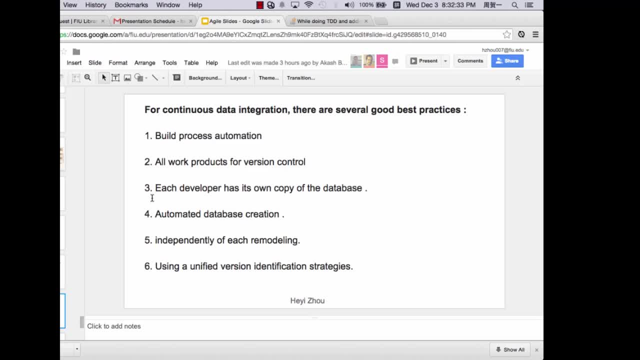 And then build scraps For continuous data integration. there are several good best practice- All of these is an example for good best practice- like build process automation or work products for version control, copy of the database and auto database creation and so on. So why use the TDD? 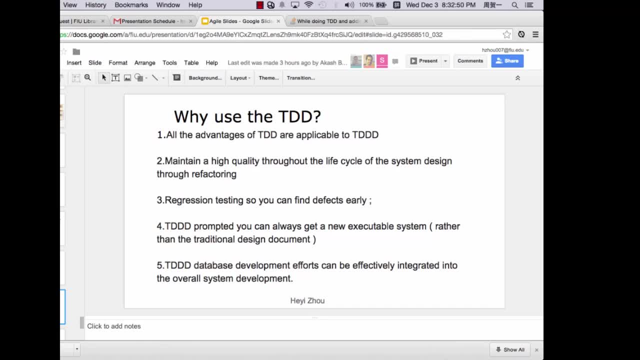 First, all the advantages of TDD are applicable to TDDD. There are five benefits for TDD users to use TDD for relational database. The first is: all the advantages of TDD are applicable to TDDD. Maintain high quality throughout life cycle. 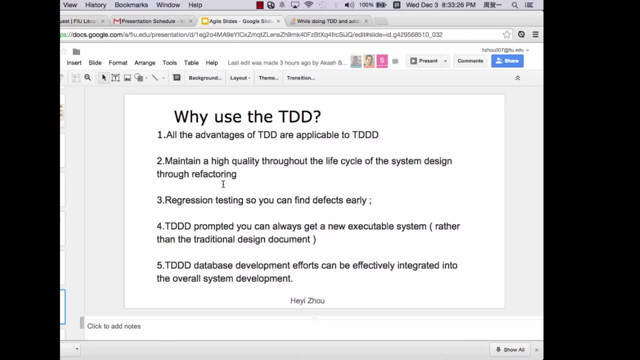 of the platform design through refactoring. Rejection testing- so you can find defect early. Rejection testing- so you can find defect. early Rejection testing- so you can find defect early. TDDD promoted. you can always get a new exactable system rather than the traditional. 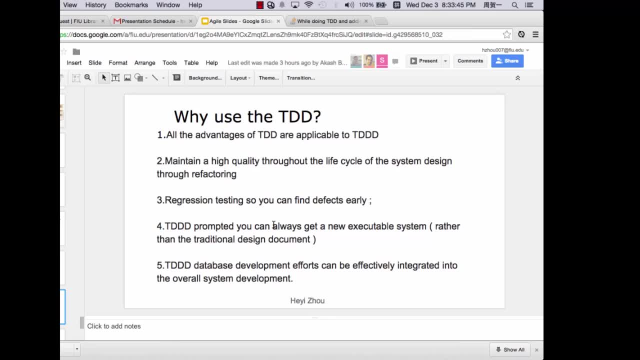 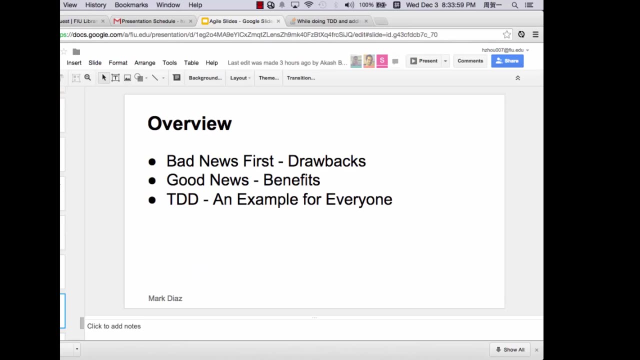 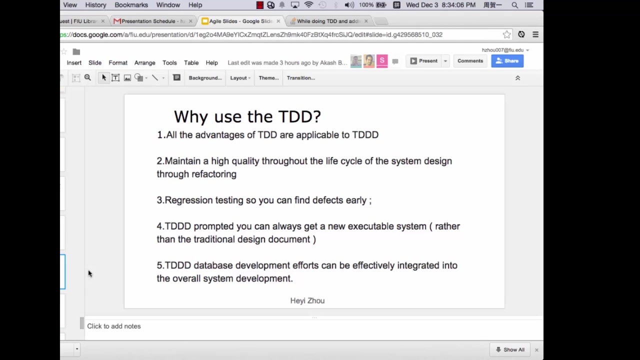 that design document TDDD database development in force can be effectively integrated into the over our system development. So, OK, I have finished my second part. The third part, Mark. we need to introduce the second part, Thank you. OK, I have finished my second part. The third part, Mark. we need to introduce the second part, Thank you. 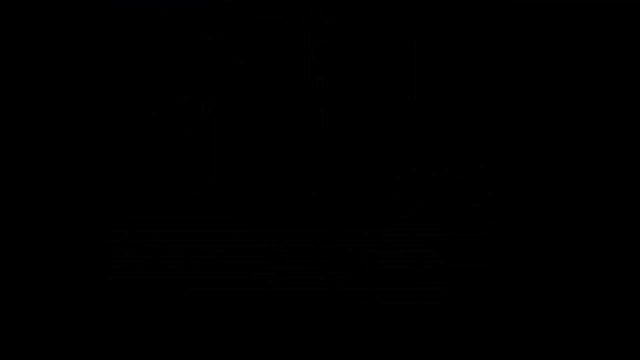 OK, I have finished my second part. The third part, Mark, we need to introduce the second part. Thank you, Hello. my name is Mark Diaz. I'm here to talk to you about test-driven development, especially the overview of it, as in the general drawbacks, benefits and an example that everyone can understand. 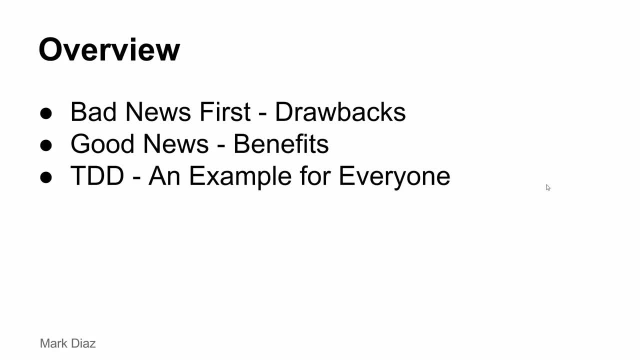 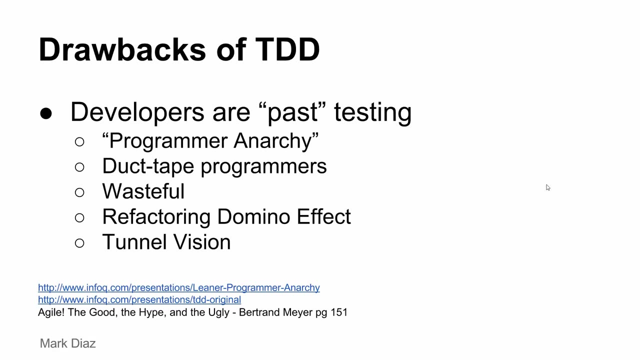 Hello, my name is Mark Diaz. I'm here to talk to you about test-driven development, especially the overview of it, as in the general: drawbacks, benefits and an example that everyone can understand. So let's jump right in. drawbacks of TDD: A lot of people aren't for TDD. They list, you know, some developers say: 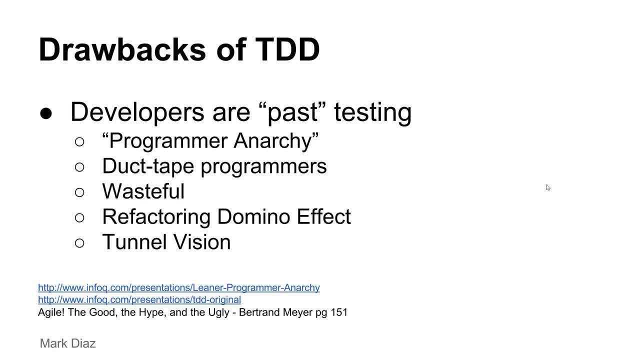 they're not testers. There's the whole programmer anarchy movement going on. You know we have people like duct tape programmers. Some people say that just testing in general is wasteful or that the domino effect from refactoring is too costly, And some people say that it has tunnel vision. I 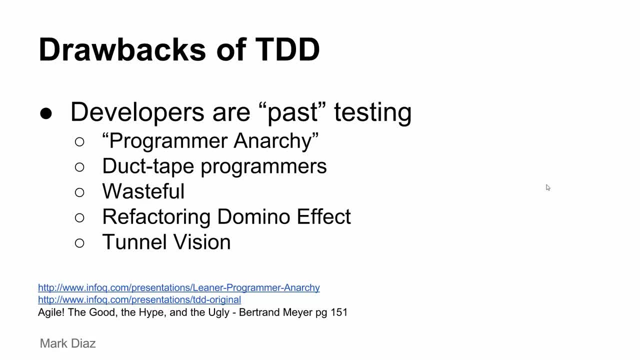 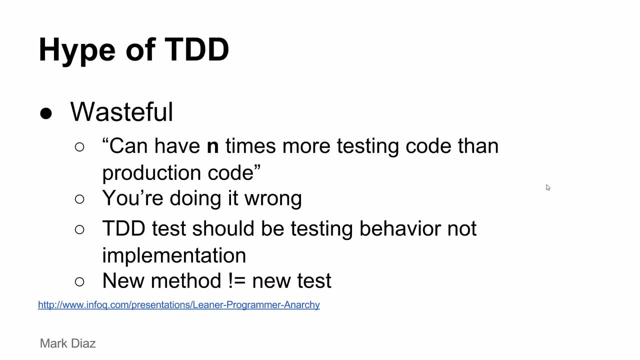 know this was mentioned in a presentation before mine, But that's all hype, Let's go into it. Wasteful. You know the common quote is: can have n times more testing code than production code. Well, that's, you're testing poorly. really is what that is. TDD testing should test behaviors. 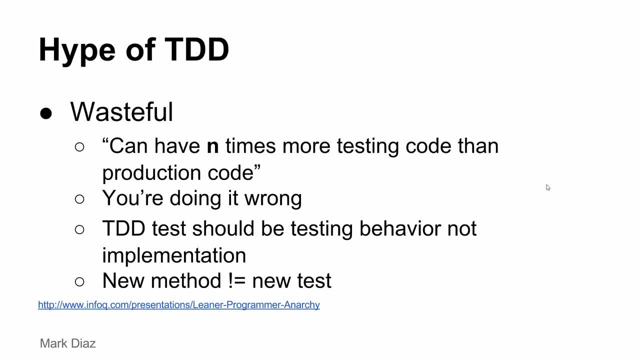 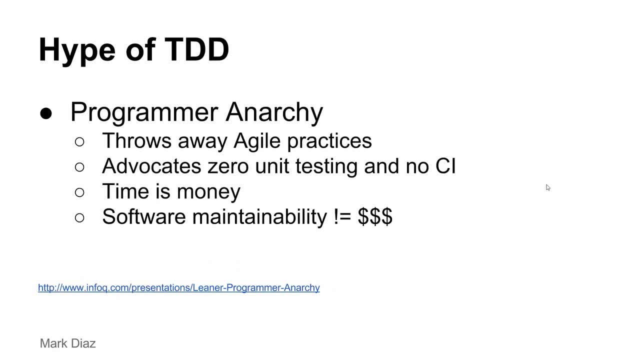 not implementation. So a new method doesn't mean a new test. You should not have all that much testing. code not n times. Programmer anarchy is a movement championed by Fred George And they throw away the idea of using agile practices like unit testing, acceptance testing, refactoring, patterns, continuous. 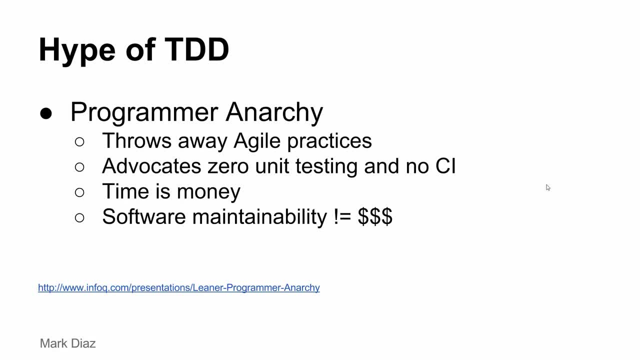 integration and more. It's pretty extreme. It's a very extreme form of extreme programming, I would say. But my general takeaway and observation is that they equate time as being equivalent to money. They don't want to talk to business analysts. They don't want to talk to 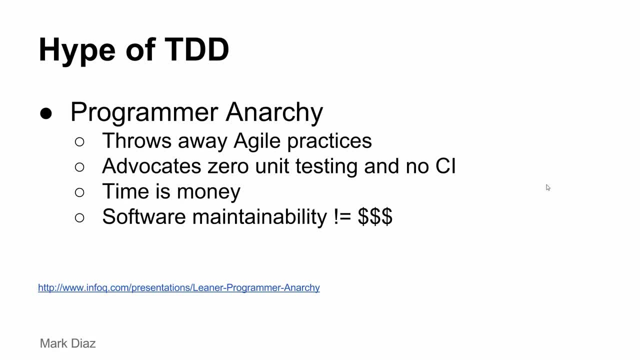 anyone but the customer And they don't feel that software maintainability is worth putting time into, therefore worth money. I guess they don't get paid to maintain software, They only get paid to create it. That seems a little bit like it's, you know, a bunch of children at the playground with no adults. 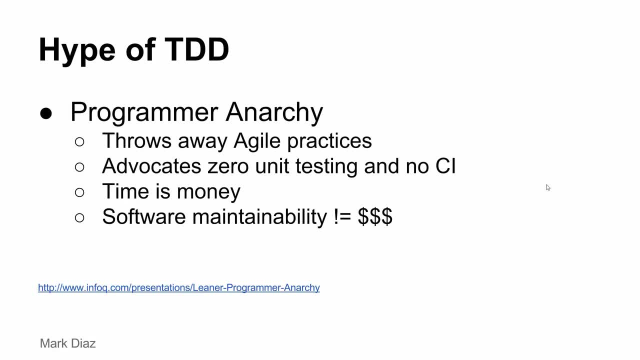 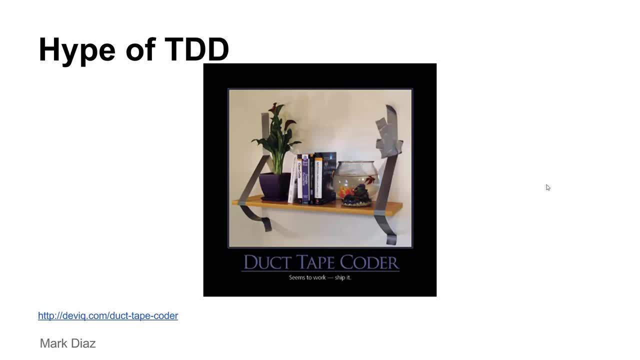 around. Or, you know, perhaps everybody who practices programmer anarchy is just a rock star Duct tape coders. It seems to work, so ship it. You know that does qualify as a shelf, Or I would not trust my fish on that shelf. 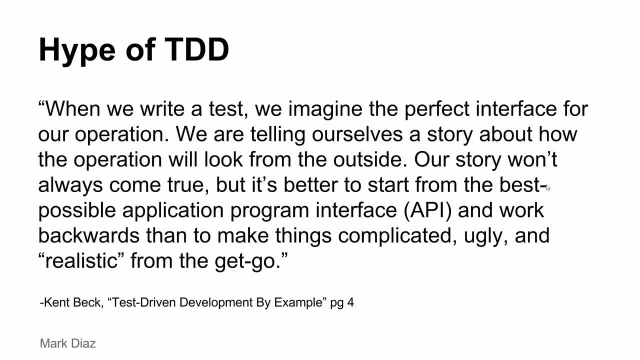 And you know, Kent Beck has this quote in his book Test Driven Development by Example, which is a seminal work for test-driven development, And it's really how to change the idea of your mind state when testing. It says: When we write a test, we imagine the perfect interface for our operation. We are telling 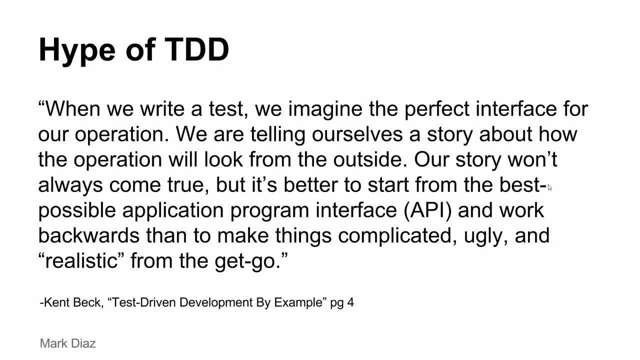 ourselves a story about how the operation will look from the outside. Our story won't always come true, but it's better to have a story about how the operation will look from the outside. It's better to start from the best possible application program interface and work backwards. 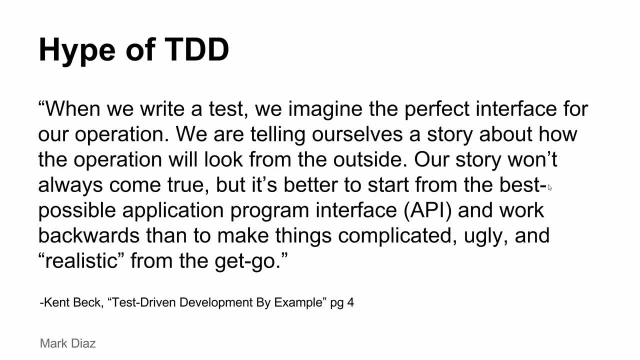 than to make things complicated, ugly and realistic from the get-go, You know. so start greenfield testing. Does this work, Doesn't this work? And then you'll take the exceptional flows as they come. That being said, you know there is what is perceived as being the refactoring. 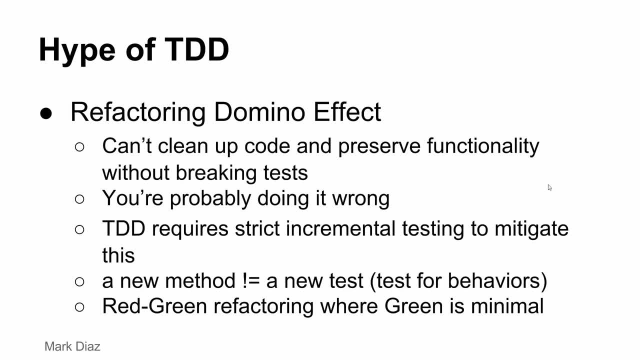 domino effect. People claim they can't clean up their code and preserve functionality without breaking tests. Well, if that's the case, they are also refactoring incorrectly. Refactoring has the idea of not changing the behavior of the code, And since TDD should. 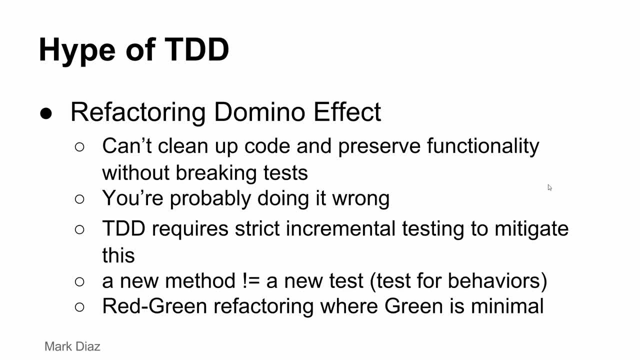 be testing for functionality that shouldn't be impacted at all. TDD also has set rules, and those require strict incremental testing to mitigate this. So you should be refactoring after every green test, assuming that it is necessary Once again. a new method doesn't. 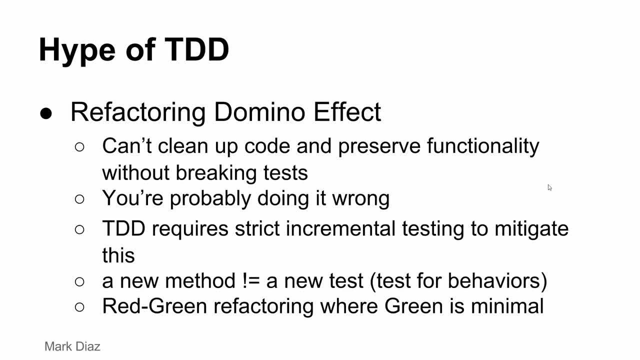 equal a new test And you know it's red-green. refactoring: Refactor as soon as possible, As soon as it's green, And then go back, start a new test and you're red again. TunnelVision was listed as being a drawback for test-driven development, but I just 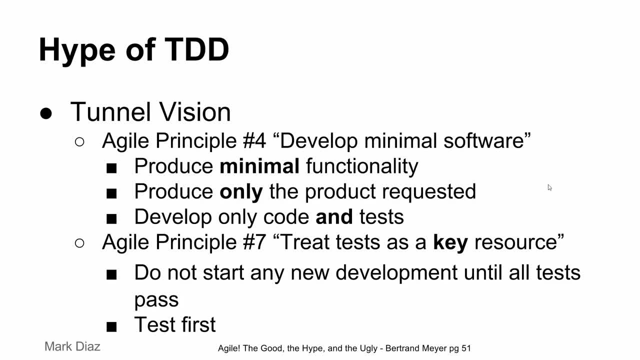 found that somewhat ridiculous, As Agile Principle number four says: develop minimal software, which implies produce minimal functionality. Produce only the code, the product requested. Develop only code and tests. Agile Principle number seven says: treat tests as a key resource. Do not start any new development until all tests pass. and 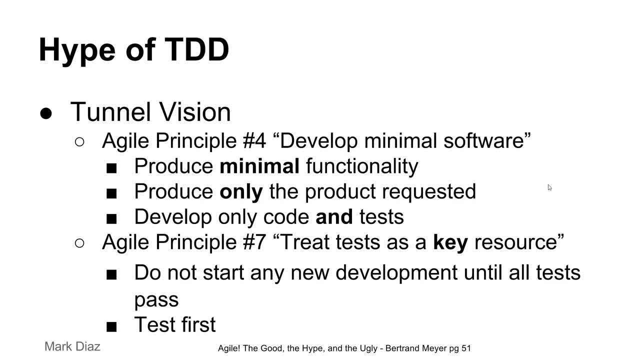 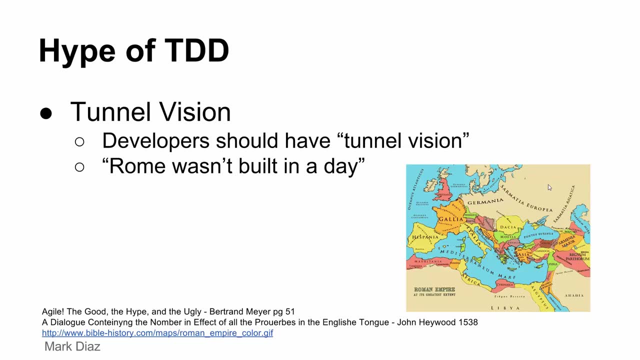 test first. These are verbatim from Agile- the Good, the Hype and the Ugly by Bertrand Meyer and are strongly in line with test-driven development. So I don't necessarily see that there's a problem or even a disconnect here. This is full go. Developers should have TunnelVision. 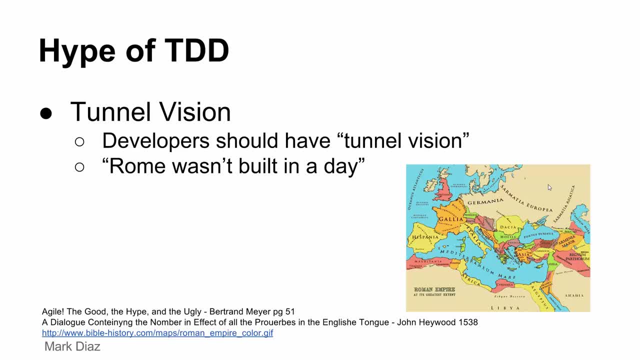 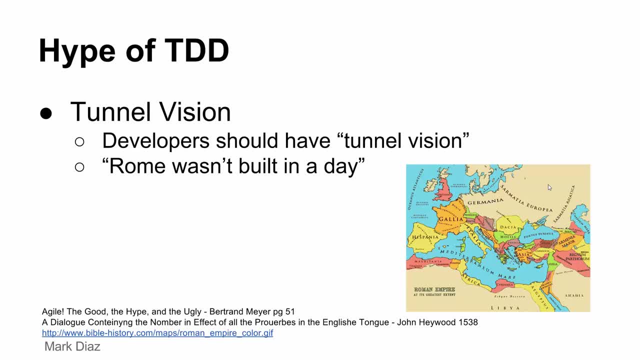 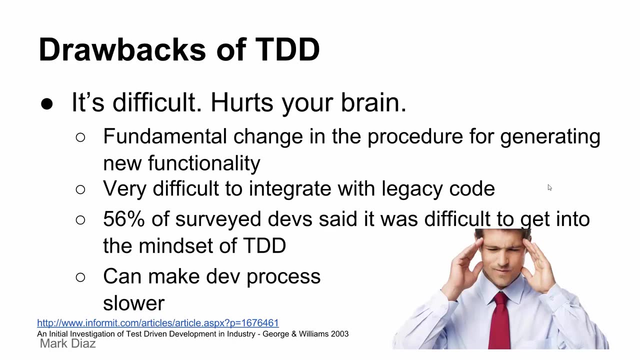 of years to conquer all of that territory and it was all done piece by piece. just like complicated software is done Piece by piece. it takes time, but if every piece is done correctly it will work correctly. There are some actual drawbacks of TDD and it's commonly noted that it is difficult. 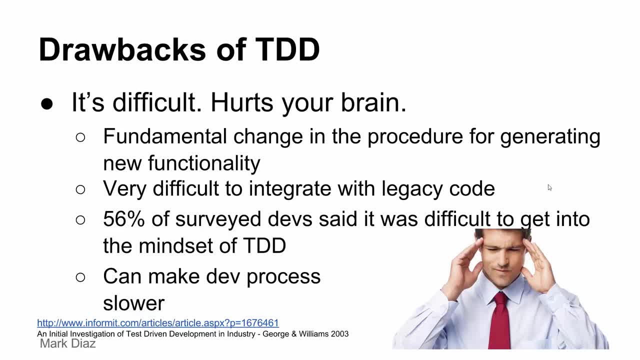 It's a fundamental change in how you think about your code, how you go about writing your code. Everybody has their own style, their own way of writing their code, their own thought process, And this is imposing a strict procedure on that a bit. It's also very difficult to integrate. 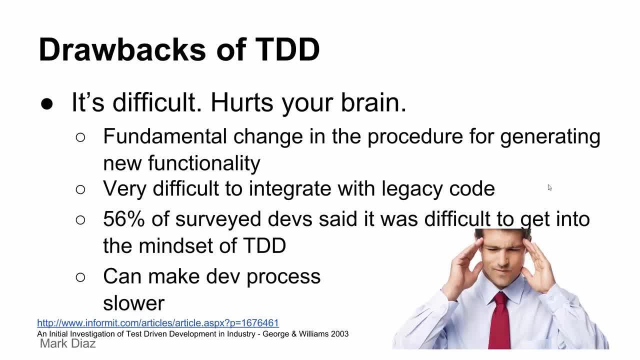 with legacy code, because the functionality for legacy code may not have been tested already, So now you have to go back and implement those tests as well. Surveyed developers: 56% of them said it was difficult to get into the mindset of TDD and 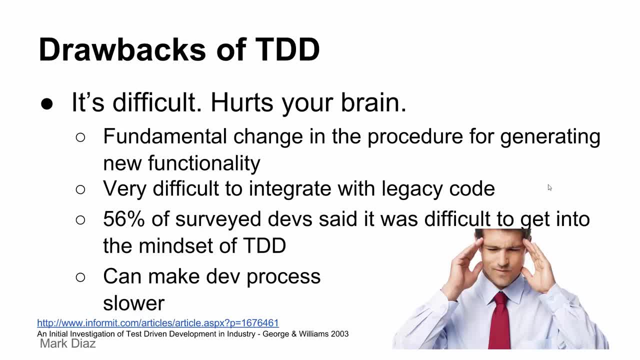 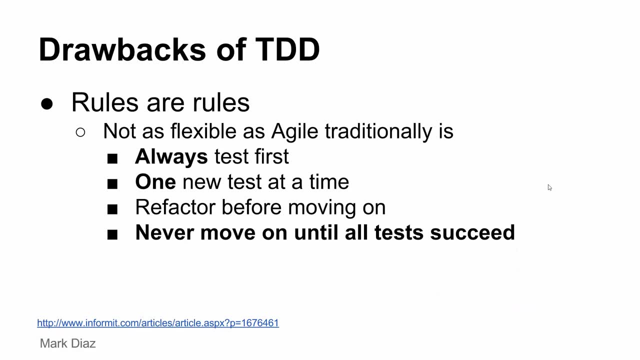 it has been observed to make the development process slower, But that was mostly for studies done with companies new to TDD And it could be that, you know, with time and practice it becomes more natural. TDD definitely has rules. You know the rules are always: test first, one new test at a time, refactor before moving. 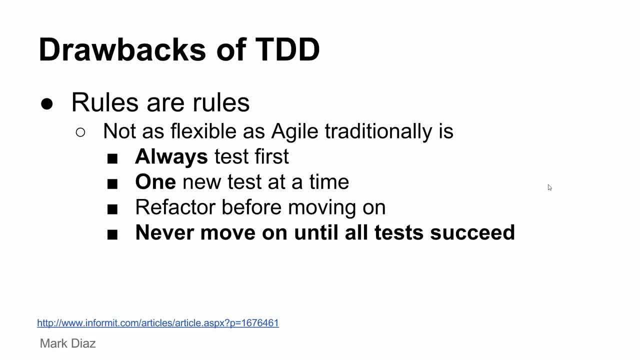 on and never move on until all tests succeed. It's the incremental nature of that that will help you catch problems, fix issues and refactor. well, You know, just like Fight Club, the first rule of TDD is: rules are rules. You know, just like Fight Club, the first rule of TDD is rules are rules. 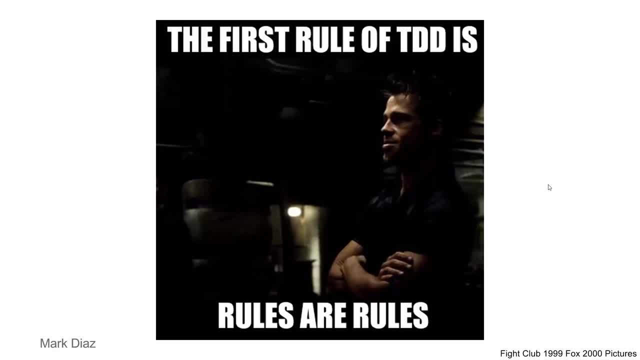 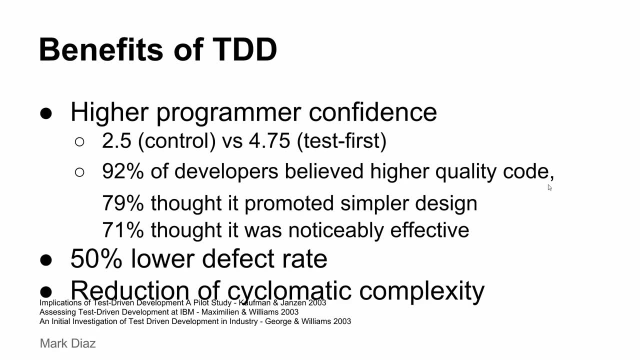 You know, just like Fight Club, the first rule of TDD is: rules are rules, And it's also the second rule of TDD. There are some benefits to TDD: Higher programmer confidence on a scale of 1 to 5.. 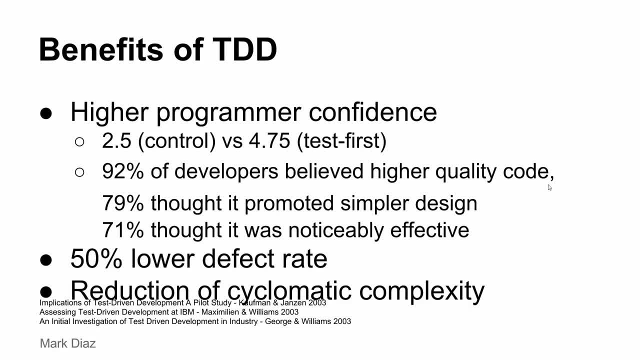 The control group rated their confidence in their code at 2.5, whereas the test first group rated it at 4.75.. Out of surveyed developers, 92% believed that TDD created higher quality code. 79% thought it promoted simpler design. 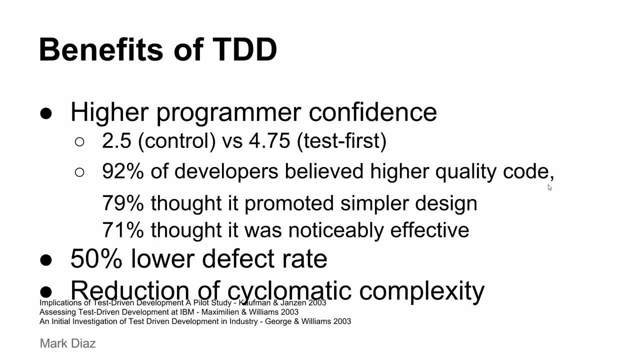 71% thought it was more efficient. 72% thought it was noticeably effective. There was an observed defect rate that was 50% lower than the control group, And there is a reduction of cyclomatic complexity, because the code developed should be simpler. 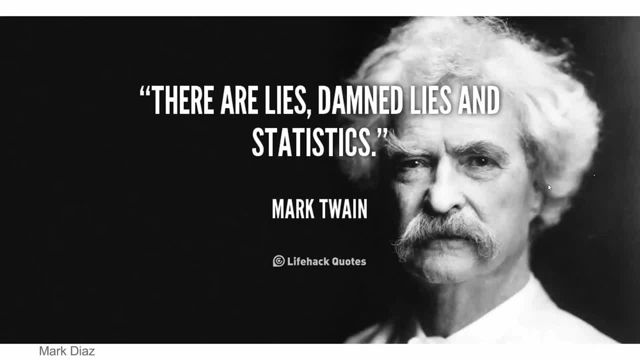 and more direct. But then there are three kinds of lies. There are lies, damned lies and statistics. That previous slide was purely statistics and you can spin those however you like. The surveyed devs were not the devs on your team. They were not even the devs of your company. 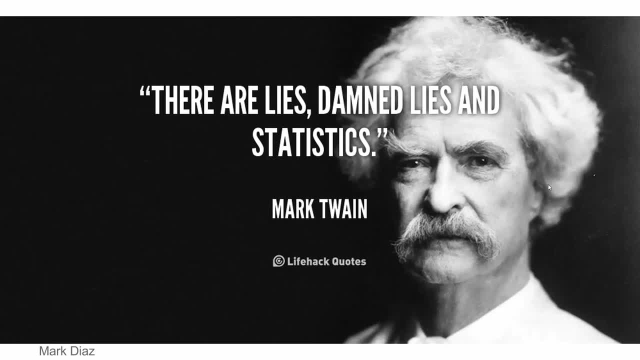 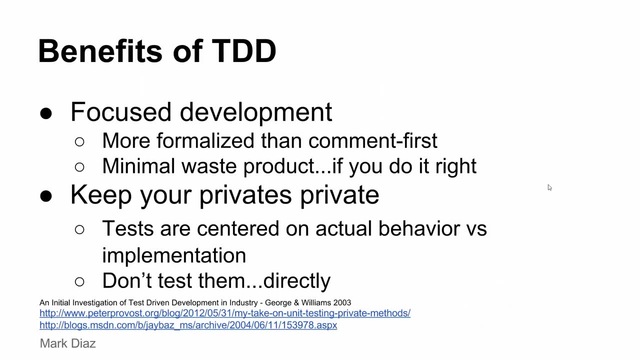 So it's going to be different for everybody, but there are potential drawbacks and benefits for everything. So you know, a legitimate benefit of TDD is that there is focus development. It's like comment first, which Dr Sajjadi mentioned. 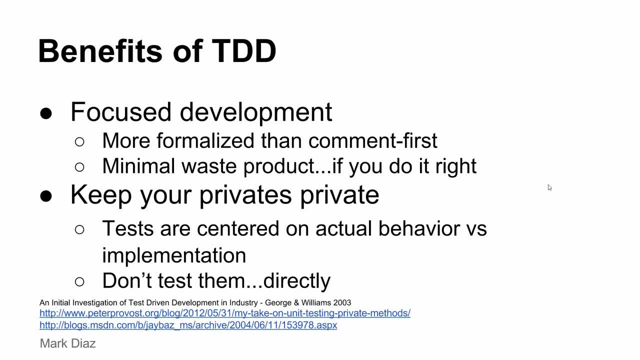 It's just more formalized. You have, you know, tests that pass and tests that fail, And then there's minimal waste product. if you do it right, You won't have pointless tests, you won't have pointless classes, pointless methods. 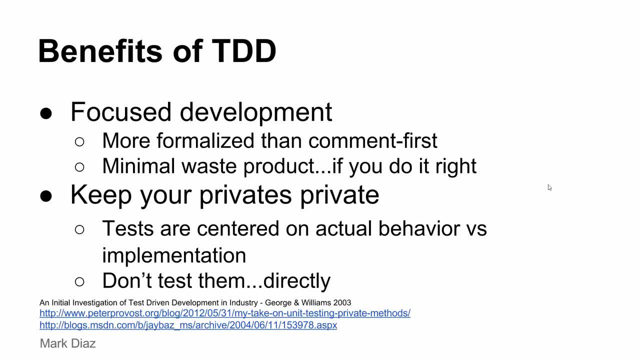 You're also able to keep your privates private. The tests are centered on behaviors that the user will see or interact with, as opposed to the return value of each method, So you don't have to test your private methods directly. You know there have been blog posts and developers who say that there should be no private methods. 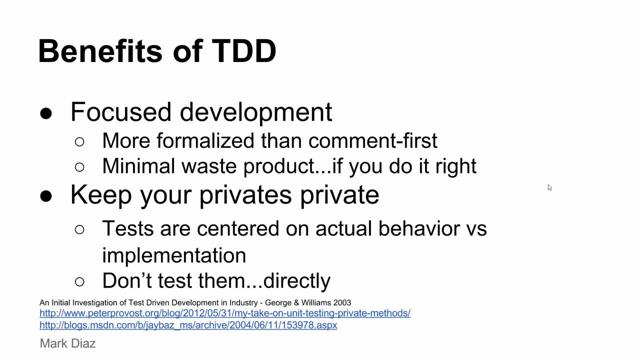 at all ever, Because private isn't really private and you know, one of their rationalizations is that if somebody wants to access your private method, they can hack your program and do it anyway. But that's not necessarily valid, because it's about compartmentalization and information. 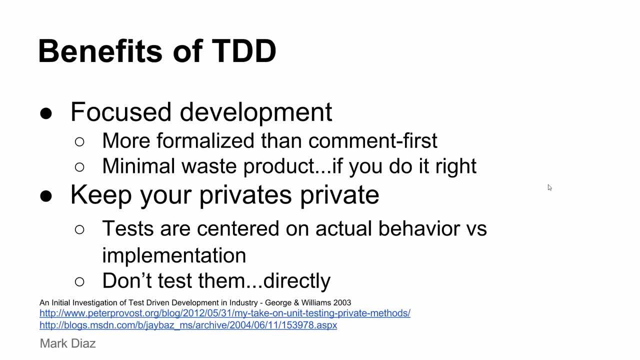 hiding. You know, in a Greenfield case you don't have to assume that everybody's going to hack every program. So you don't test your privates directly with TDD, but you do only develop the minimal code necessary. So the privates that you do have are necessary for end functionality, which means that your 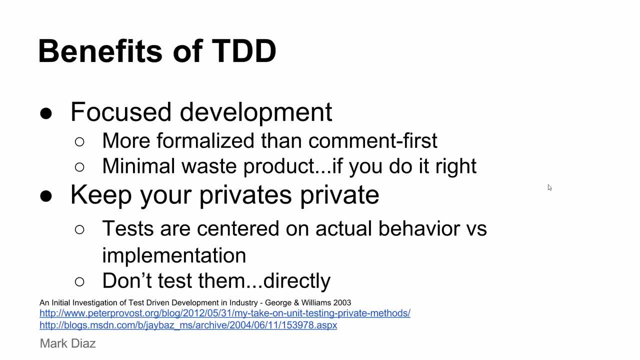 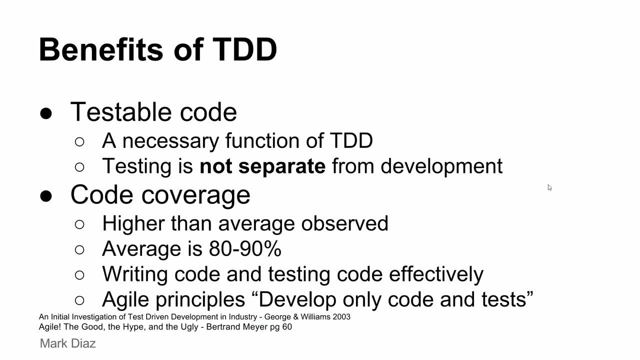 functionality testing or your- you know, basic tests are going to test your private methods. Your code is now by nature, going to be testable. Testing is not separate from development at all. Testing is a key resource in the Agile manifest or in Bertrand Meyer's summarization of the. 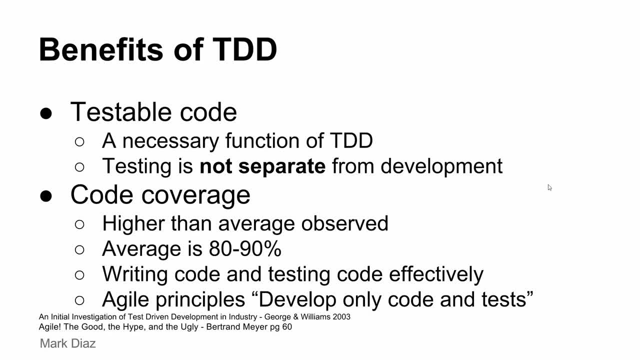 Agile principles. You know there is going to be a higher than average code cut. Code coverage averages 80 to 90%. as far as testing, You're going to be writing code and testing code effectively. So even though you may be writing a few, you know less lines of code per month or whatever the metric that your team or company may use. that code should be more effective. 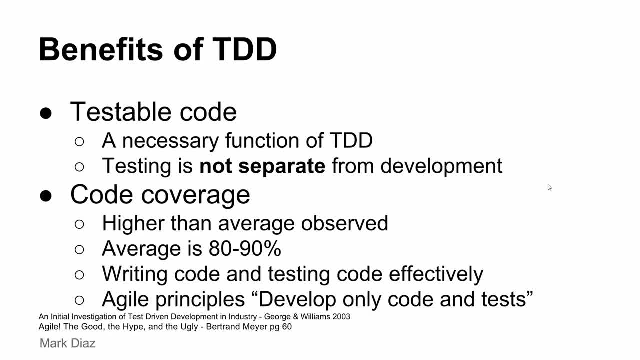 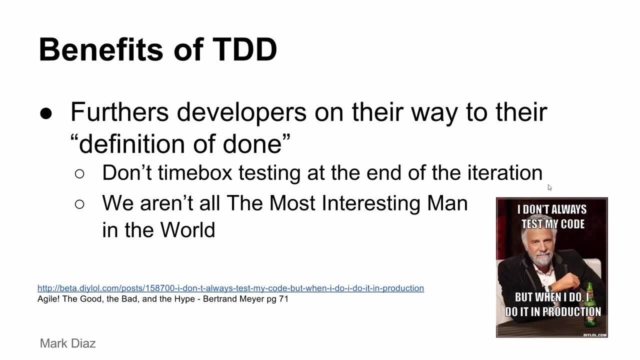 It will definitely be used in the product and it definitely has functionality and purpose. Agile principles are develop, only code and tests. Testing is always what gets cut. Every time something's on a deadline it's like: oh, cut testing, just ship it. 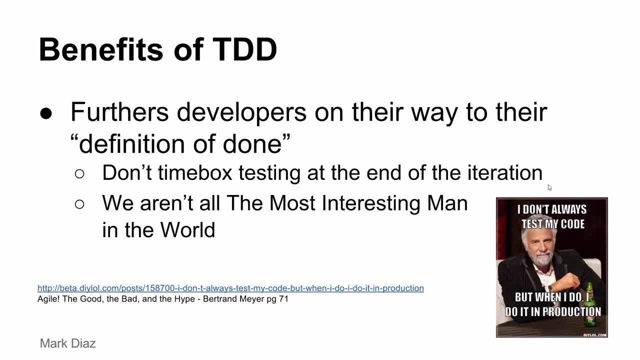 But through TDD you by nature cannot time box testing at the end of the iteration. We should all test our code. We are not, you know all, the most interesting man in the world. We're not perfect, So please test your code. 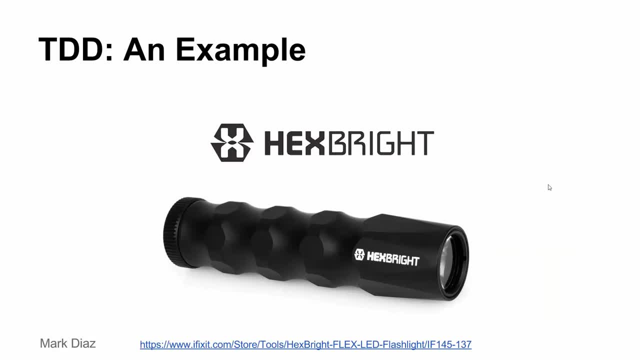 For an example that everybody can understand, I'm going to talk about a flashlight. This flashlight I actually own. It's a Hexbrite. It's a fantastic device and I purchased it through its Kickstarter. It has some really cool functionality, but let's go through it as if it had not been implemented. 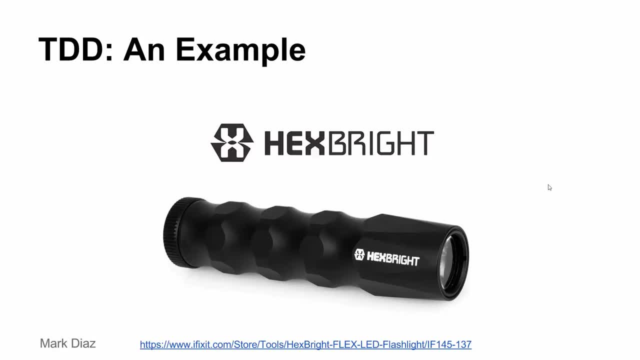 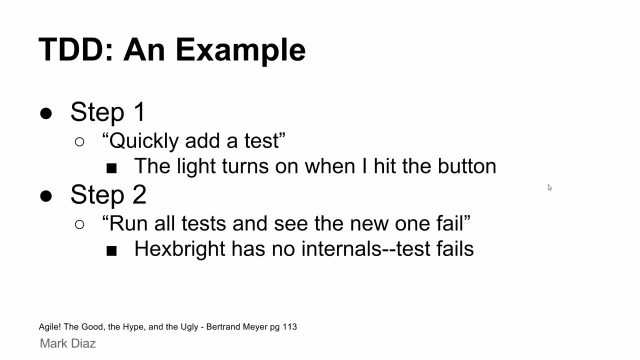 You know, let's just assume that we have the shell that you see here and the button has one single button on the back. So in TDD, step one is quickly out of tests, Right? So my test is going to be that I want the light to turn on when I hit the button. 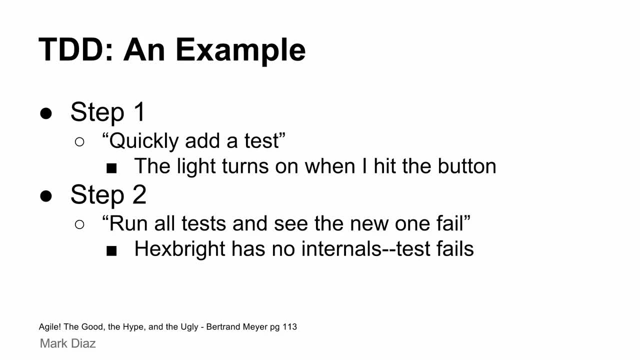 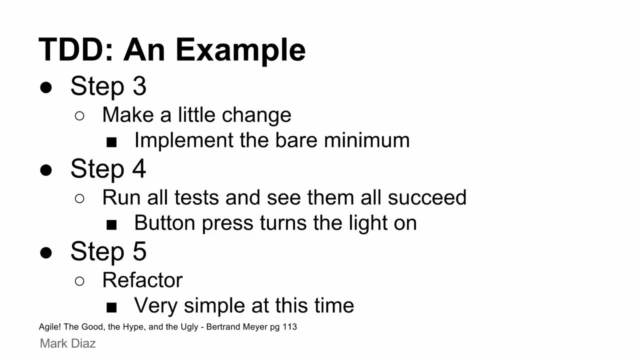 Step two: I'm going to run all tests and see the new one fail. Well, we only have one test and it's going to fail As the Hexbrite has no internals. Step three is make a little change. So we're going to implement the bare minimum: a battery, a circuit that will, you know, take the current from the battery and, you know, provide light from the LED. 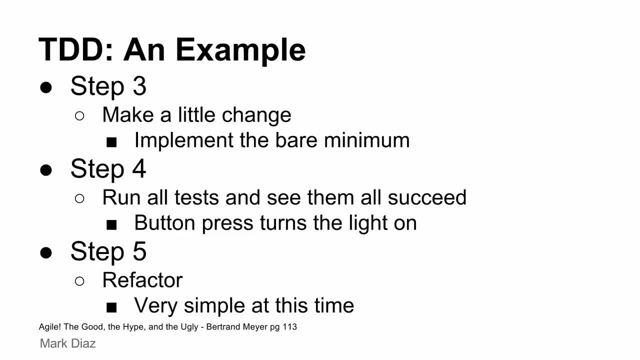 And the internals of the button, I suppose the switching part of the button. So now step four. we're going to run all tests and see them all succeed. press a button and the light turns on. We have one test. That test is now green. 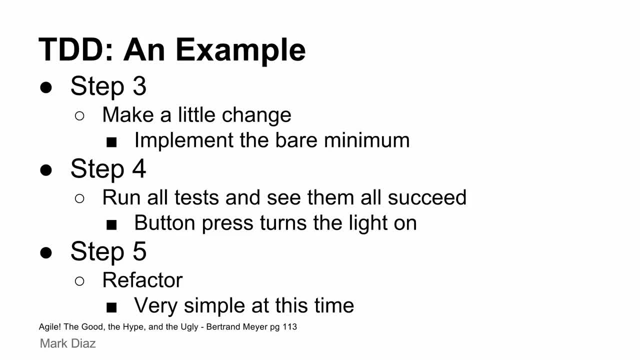 Step five is refactoring. However, everything is very simple at this time, but we don't necessarily have to refactor everything. It's a button, a small circuit and that's about it really. I mean cause the LED would be part of the circuit. 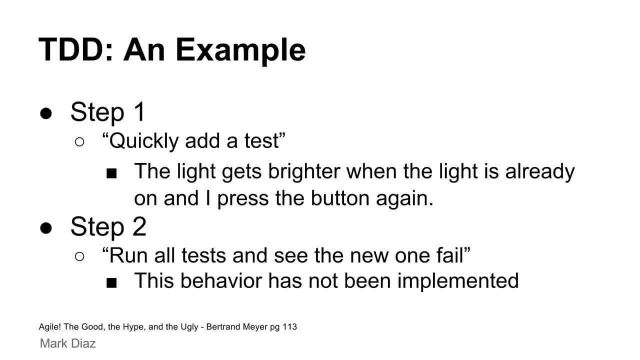 Then we're going to go through the second iteration, which is quickly out of tests. We want to add a second stage of brightness where the light will get brighter If the light is already on and I press the button again. Step two is run all tests and see the new one fail. 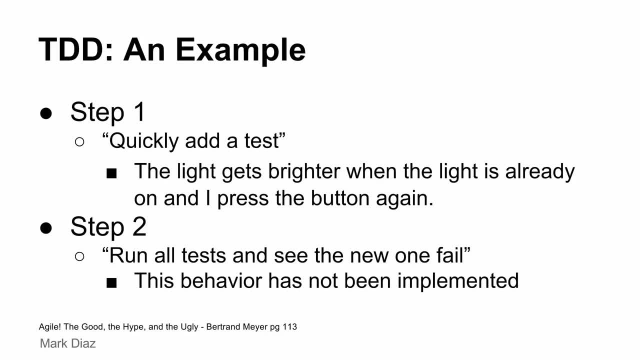 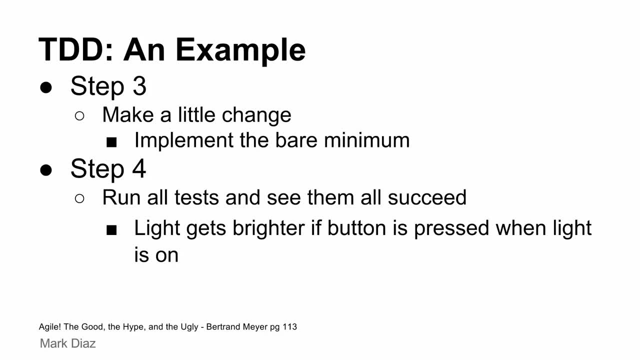 This behavior hasn't been implemented yet, so it will fail. Step three: make a little change, implement the bare minimum. This will probably require a little more advanced of a circuit, some logic in there, but then we're going to run all tests and see them succeed.